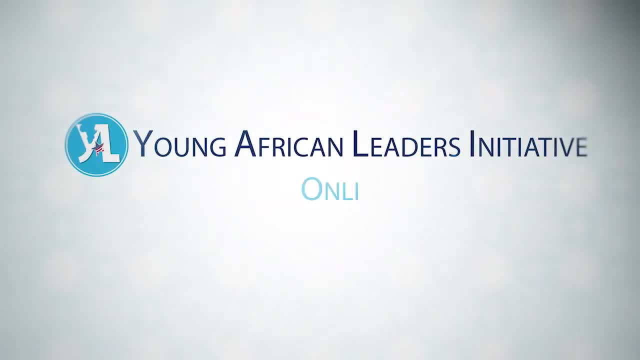 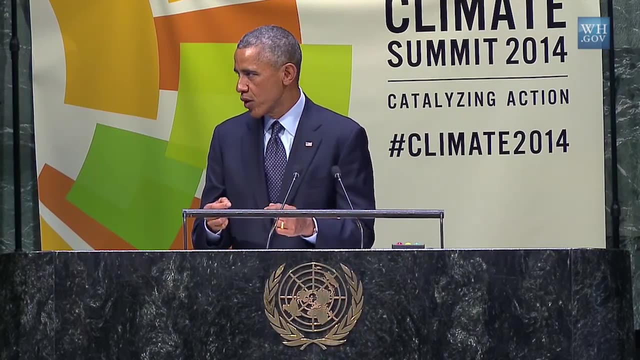 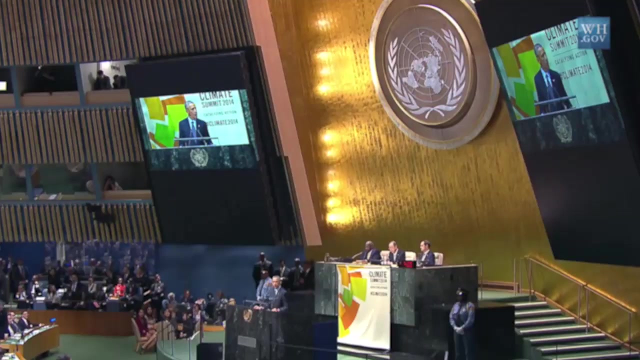 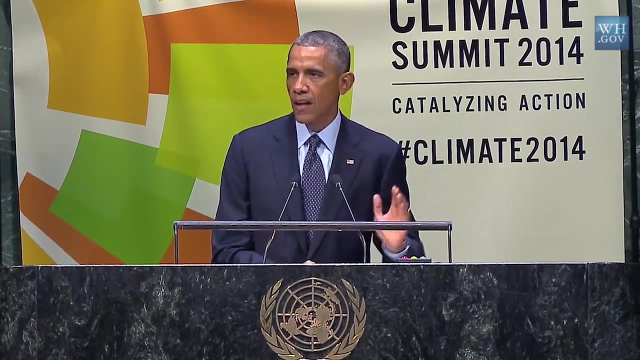 The climate is changing faster than our efforts to address it. The alarm bells keep ringing. No nation is immune. Worldwide, this summer was the hottest ever recorded, with global carbon emissions still on the rise. We are the first generation to feel the impact of 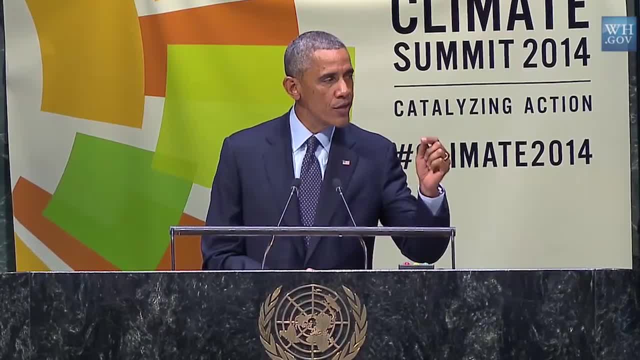 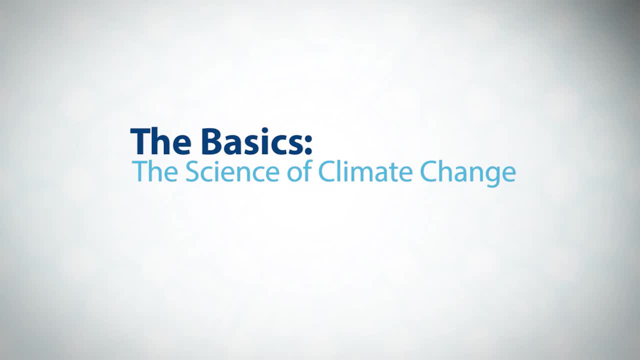 climate change and the last generation that can do something about it. We've all heard about climate change. It's in the news and on the agenda of leaders and scientists across the globe. But what is it really, And how are humans changing the Earth's? 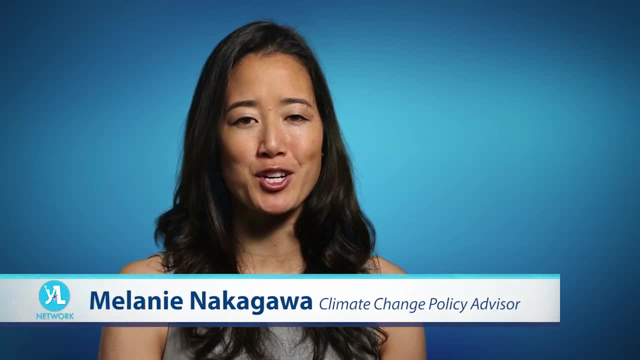 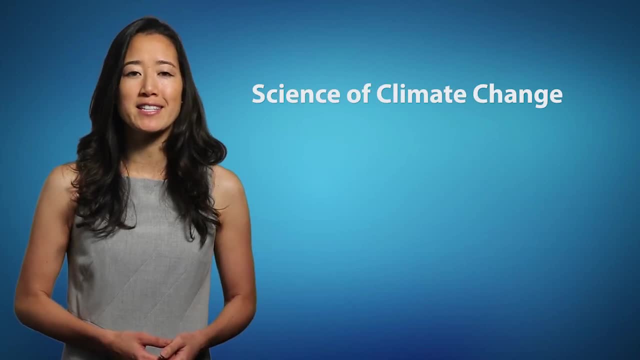 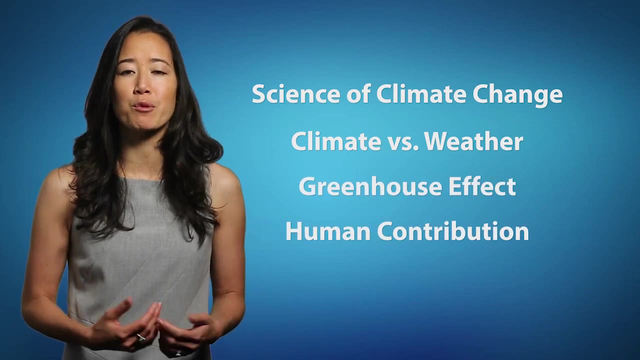 climate. I'm Melanie Nakagawa, a policy advisor on climate change to US Secretary of State John Kerry. In this lesson, we'll examine the science behind climate change, take a look at the distinction between climate and weather and learn about the greenhouse effect, including how human behavior contributes to the warming. 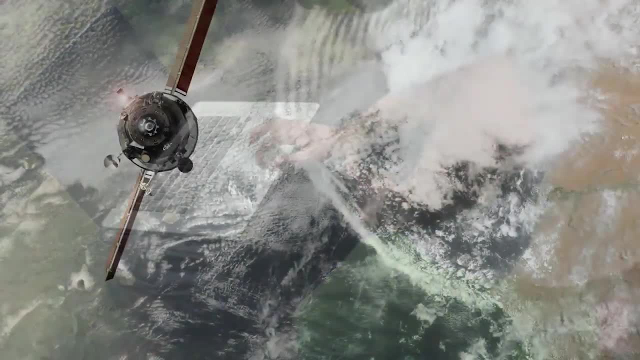 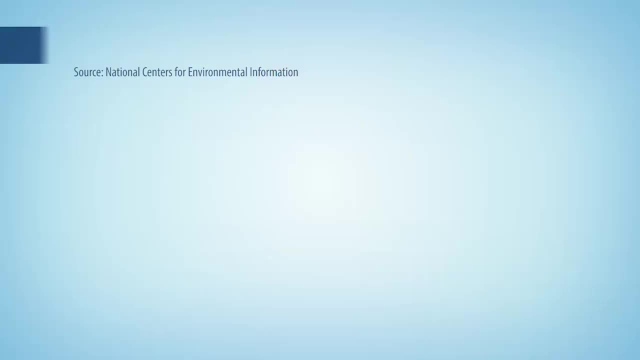 of our planet. Scientists around the world have looked at data from satellites. They've studied weather patterns and measured changes in crop yields and soil composition, And what they've found is that our planet is, on average, getting warmer. Temperatures have been rising. 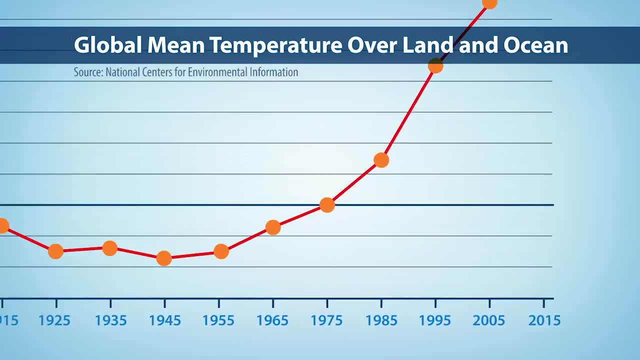 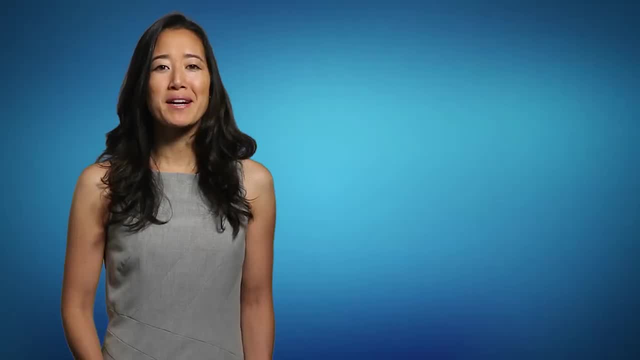 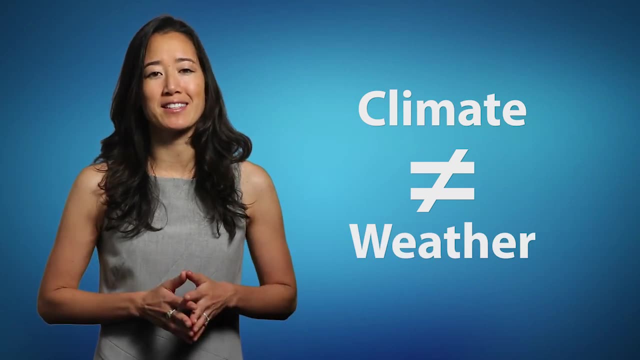 since the early 20th century and most notably since the late 1970s. This warming reflects changes to the Earth's climate, But it's important to understand that when we talk about climate, we are not referring to weather. They mean two different things. Weather can change from 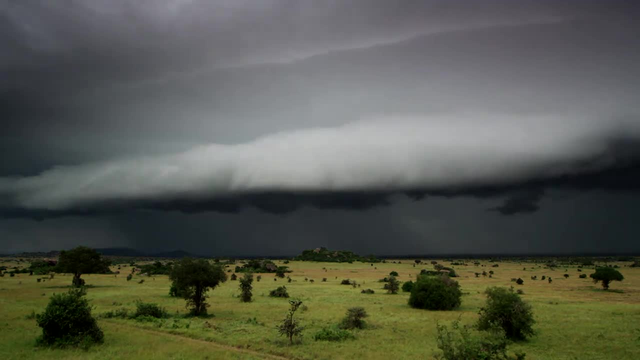 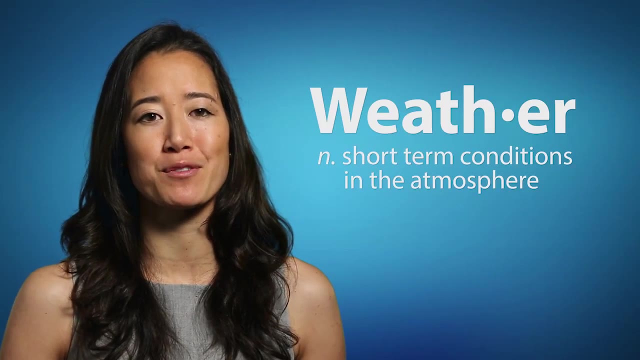 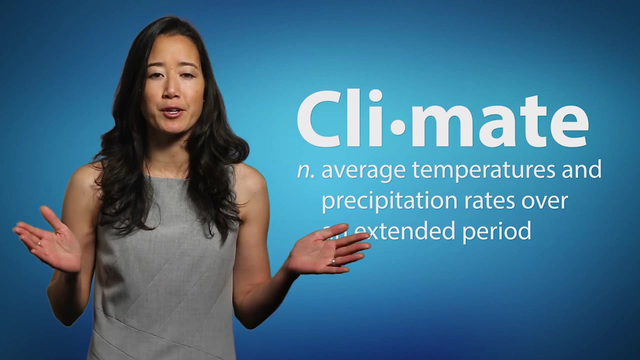 season to season, day to day, even hour to hour, sometimes when you least expect it. Weather reflects short-term conditions in the atmosphere. Climate, on the other hand, refers to the average temperatures and precipitation rates over an extended period of time, And 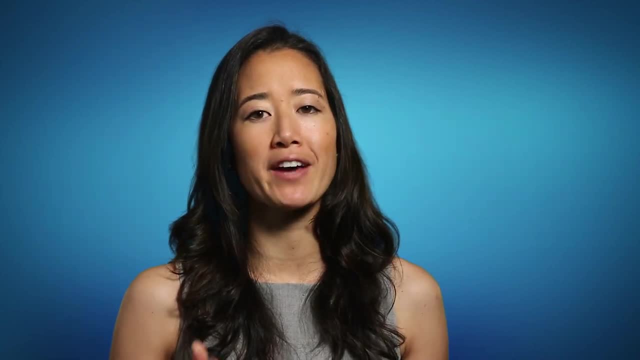 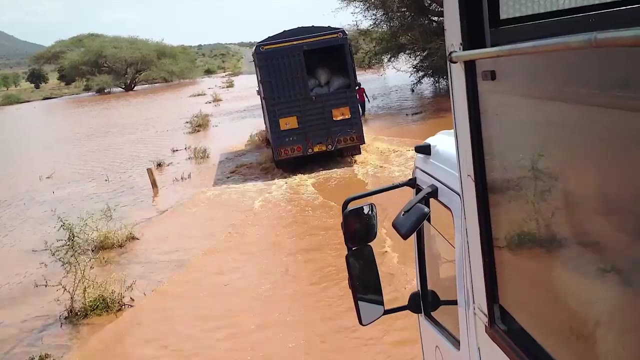 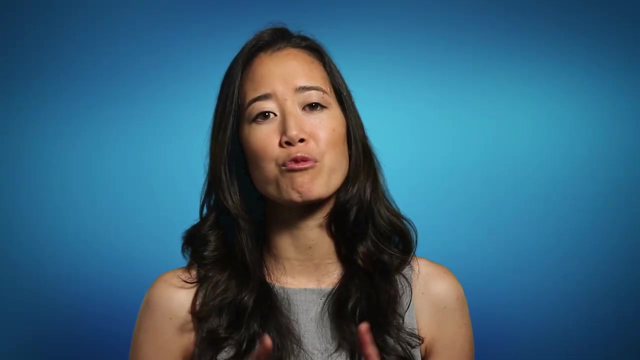 when these rates change over time, it can result in profound impacts on our planet, Impacts like rising sea levels, more extreme weather events like droughts and floods, melting glaciers, shifts in ecosystems as well as many others. In other words, real problems. 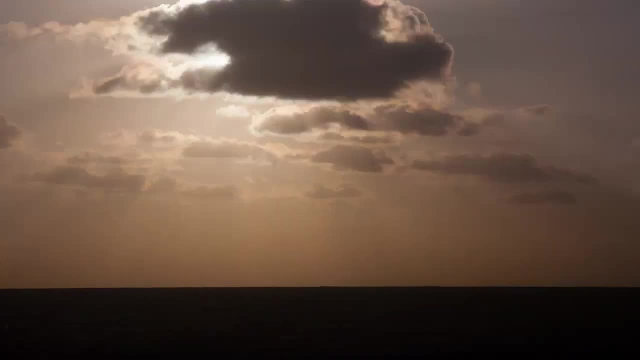 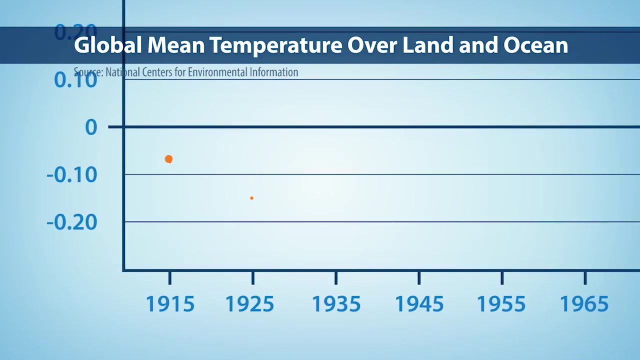 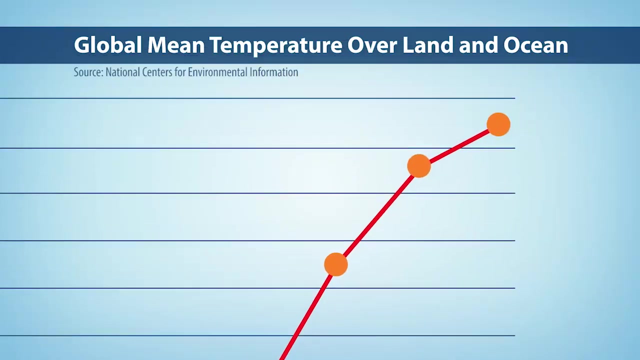 In the past, changes in our climate resulted from natural causes such as differences in the sun's activity and volcanic eruptions. However, scientists can't predict what will happen in the future. They cannot explain the warming we've experienced in the past 100 years without including greenhouse gases emitted by human activity. 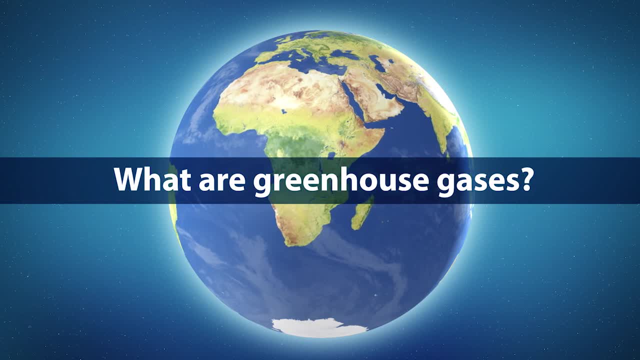 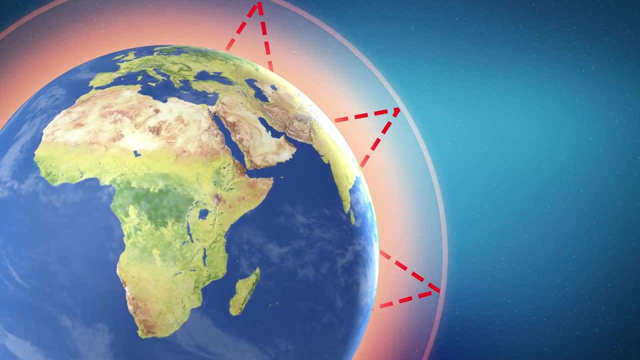 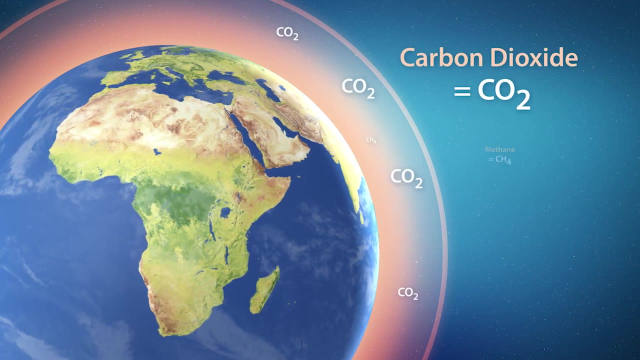 So what are these greenhouse gases? When scientists talk about greenhouse gases, they are referring to several chemical compounds found in the Earth's atmosphere which would trap heat that would normally be released out to space. Some of these compounds occur in nature, such as carbon dioxide and methane. However, others are exclusively human-made and they can be. 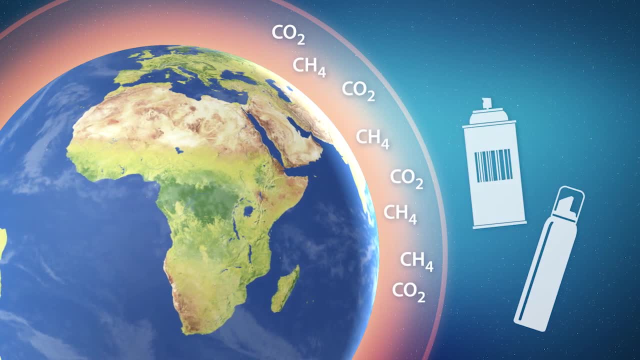 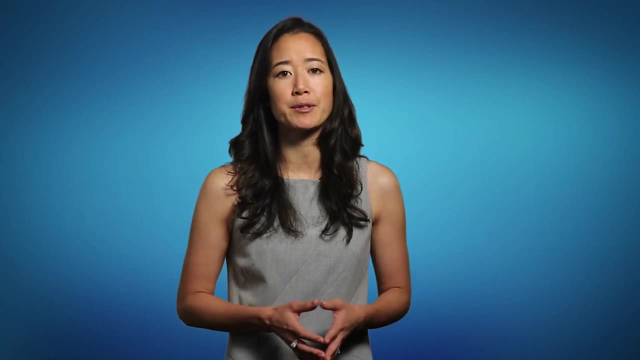 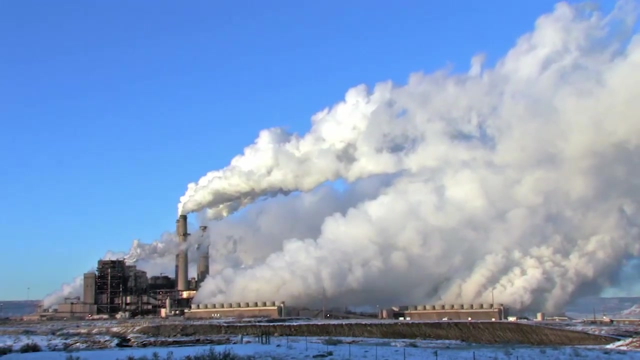 found in sources like hairspray, paint fumes and aerosol sprays. These greenhouse gases play a crucial role in warming the Earth's surface and making it habitable. However, too much human-generated greenhouse gas emissions upsets the planet's natural balance, leading 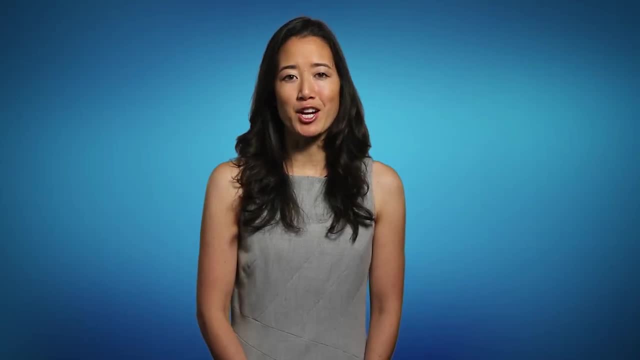 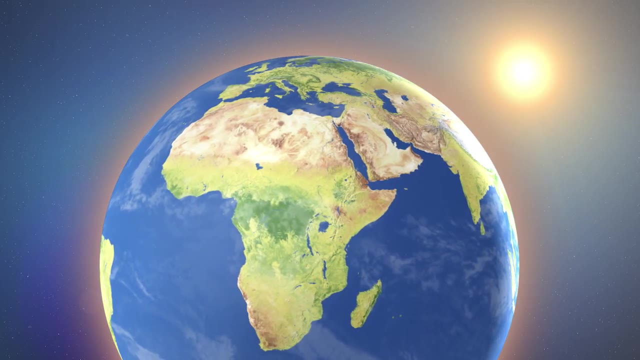 to an increase in warming. Now that we understand the meaning of climate change, let's take a look at how it actually works. Pollutants and other chemical compounds are released into the atmosphere due to human activity. The sun emits energy that is transmitted to the Earth- About 30% of the sun's energy. 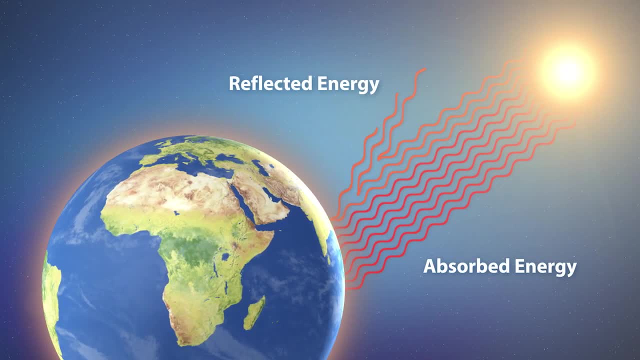 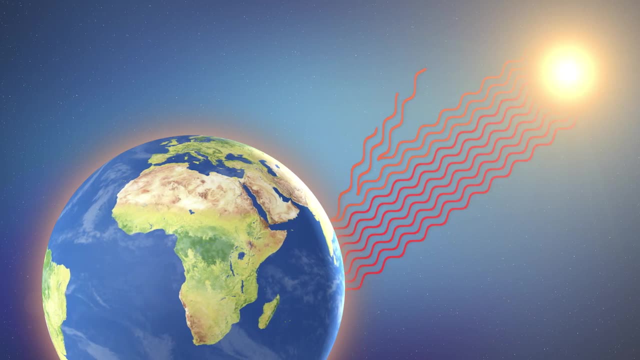 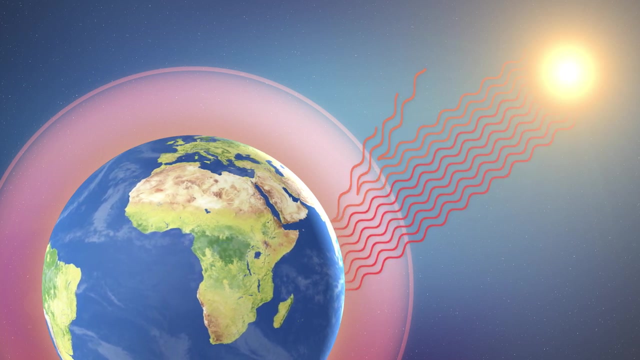 is reflected directly back into space by the atmosphere, clouds and the surface of the Earth. However, greenhouse gases in the atmosphere absorb much of the energy emitted from the warm Earth's surface, preventing it from immediately escaping from the Earth's system and back into space. 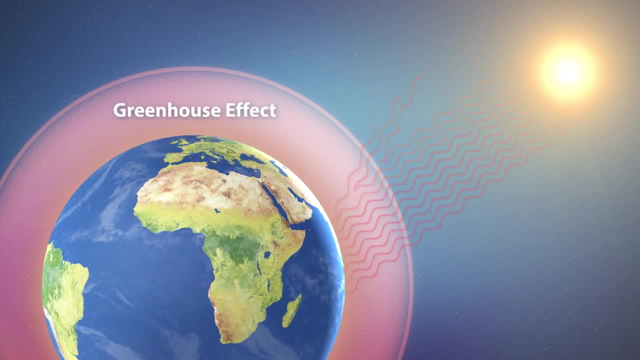 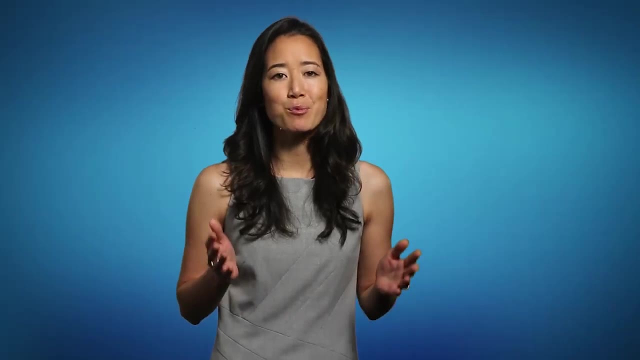 As a result, too large a concentration of greenhouse gases act like a blanket, making the Earth warmer and throwing more and more greenhouse gases into the Earth's atmosphere. Over the past 100 years, the amount of greenhouse gases in our atmosphere has been increasing. 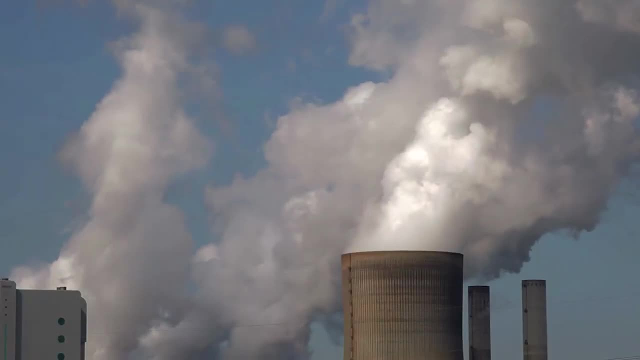 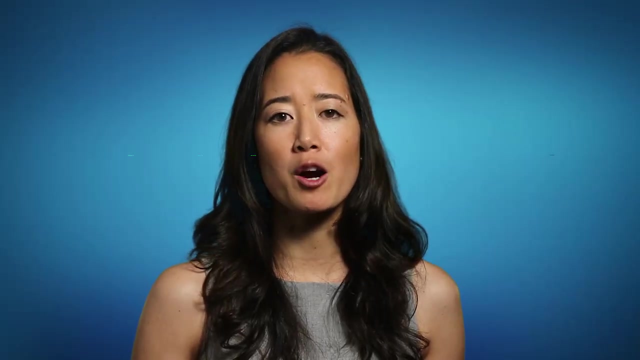 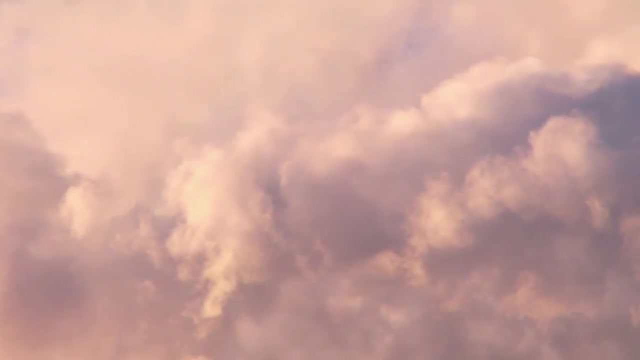 This is largely due to carbon dioxide emissions from the burning of fossil fuels such as coal, oil and gas. When these fuels are burned, carbon stored in them for millions of years is released in an instant directly into the atmosphere as carbon dioxide. Think about: